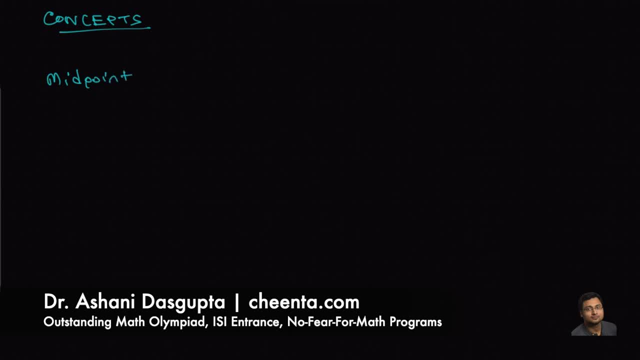 The first thing we need to learn is the midpoint theorem. We discussed this in the geometry module of Chinta Mathematics Olympiad program and the ISICMI entrance program. The midpoint theorem says that if you have A triangle, A, B, C and F, D and E are the midpoints of AB and AC. We have two conclusions. 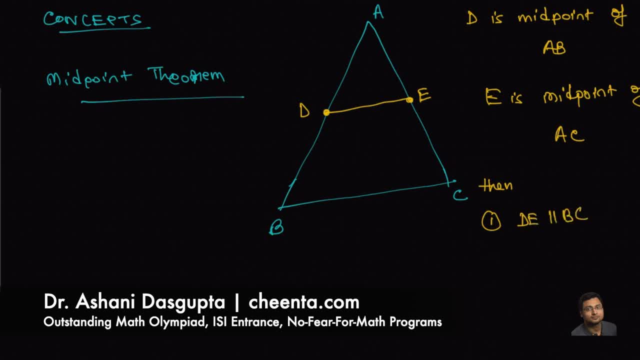 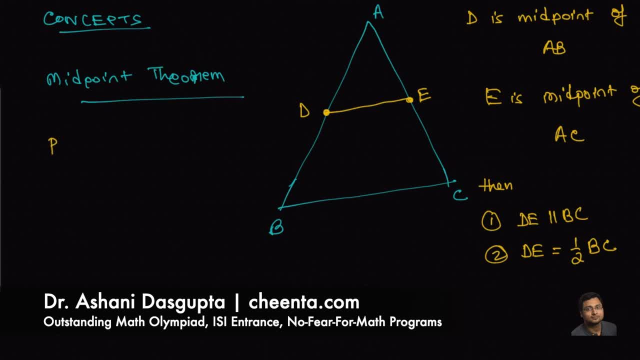 The other result that you will need is the Pythagoras theorem. You may know about the Pythagoras theorem already. It's statement is this: that you have side length A, side length B and side length C of a right-angled triangle, Then the square on the legs is equal to the square on the hypotenuse. 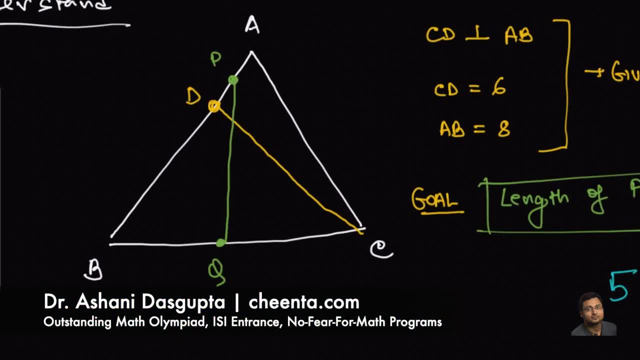 now let's get back to this diagram. we will be trying a solution of it, so first i'll give you a hint. so the hint is this: construction mark the midpoint m m of ac. m is the midpoint of ac, midpoint of ac. join pm and mq. join pm and mq. 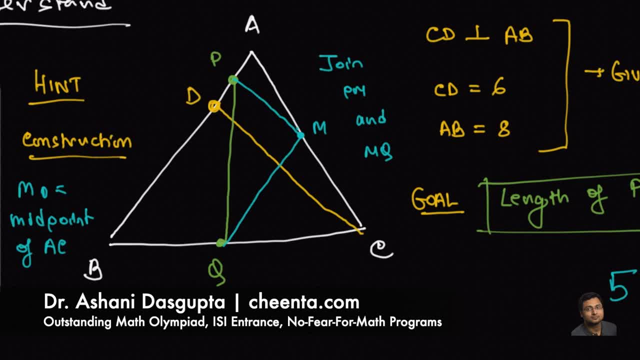 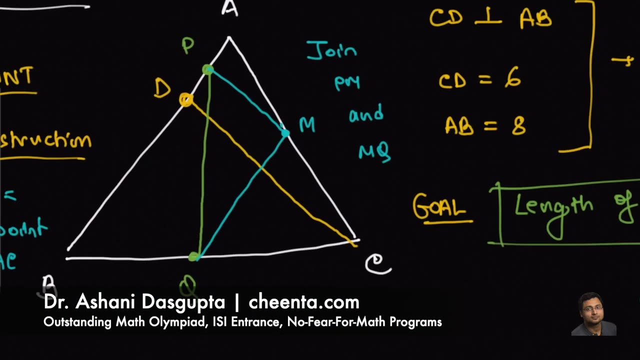 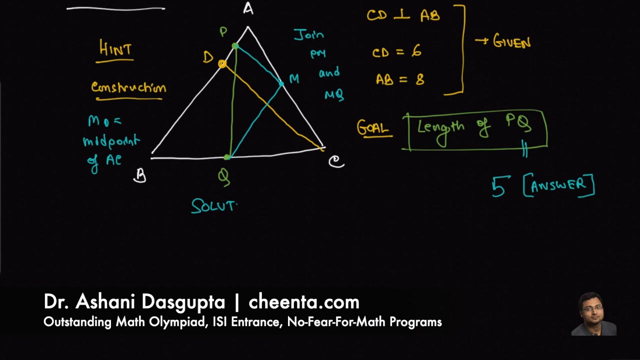 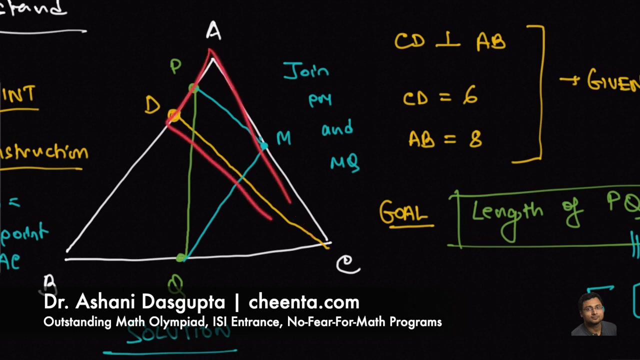 that's it. that is the hint. this construction is the hint. can you use this hint and the midpoint theorem to finish up the proof that pq is five centimeters long? you have to observe that in the triangle adc, in the triangle adc, p is the midpoint of ad, m is the midpoint of ac.